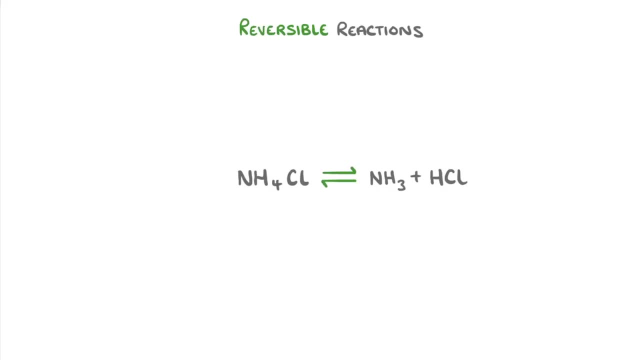 down into ammonia and hydrogen chloride, which we call the forward reaction, While the bottom arrow tells us that the ammonia and hydrogen chloride can also combine to form the carbon, to reform the ammonium chloride, which we call the backward reaction. So because both of these can happen, we call it a reversible reaction. 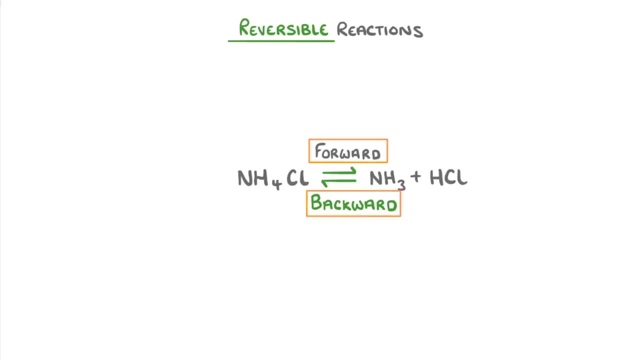 Now the important thing to understand is that the forward and backward reactions can take place at different rates. At the beginning of the reaction there'll be loads of ammonium chloride, but no ammonia or hydrogen chloride, So the forward reaction will be really fast. 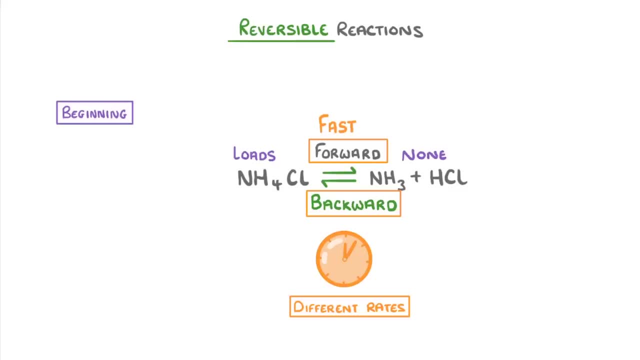 but the backward reaction won't have started yet. As the reactants turn into the products, though, the forward reaction will slow down and the backward reaction will speed up. After a while the rate will even out and the forward and backward reactions will be going at exactly the same speed. At this point, the concentrations 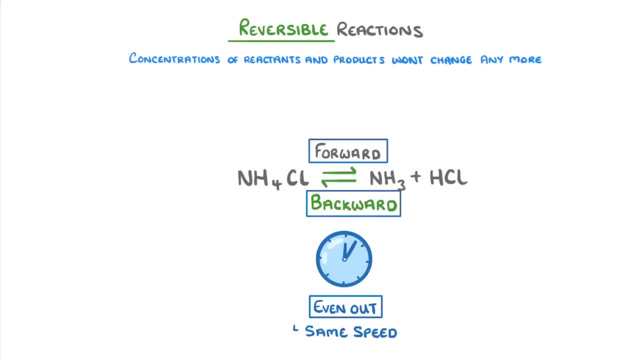 of the reactants and products won't change anymore, so we can say that the reaction is at equilibrium. So to clarify: At equilibrium Both reactions are still happening, but they effectively cancel each other out, so there's no overall change in the concentrations of the reactants or products. 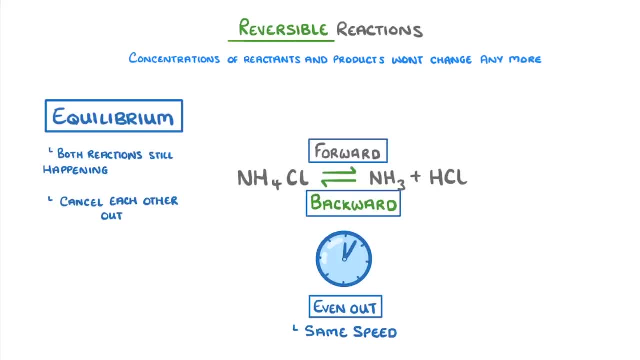 Of course, in reality, the molecules are still breaking down and reforming, but because they do so at the same rate, there's no overall change in the concentrations. Now, something to point out here is that just because the concentrations of the reactants 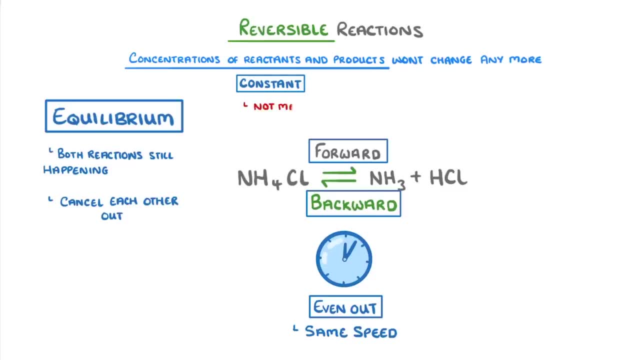 and the products are constant while at equilibrium does not mean that they're the same as each other. For example, there could be lots of ammonium chloride and only a small amount of ammonia and hydrogen chloride. Or there could be lots of ammonia and hydrogen chloride but only a small amount of ammonium. 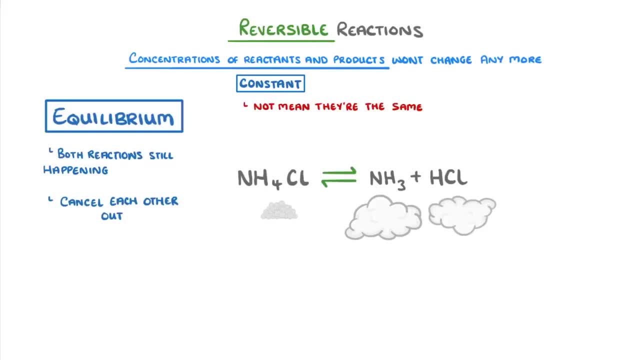 chloride. In either case, though, as long as the forward and backward rates are the same, then the reaction would still be at equilibrium. However, what would happen? What would change when we have these different concentrations, is the position of the equilibrium. 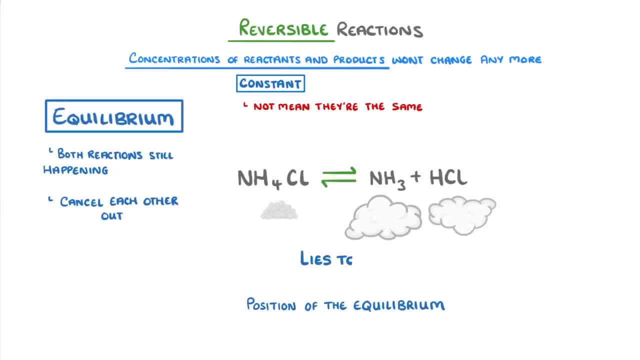 When there are more products like this, we would say that the equilibrium lies to the right. but if we had more reactants and fewer products again, then we'd say that the equilibrium lies to the left. This position of equilibrium can change depending on the conditions. 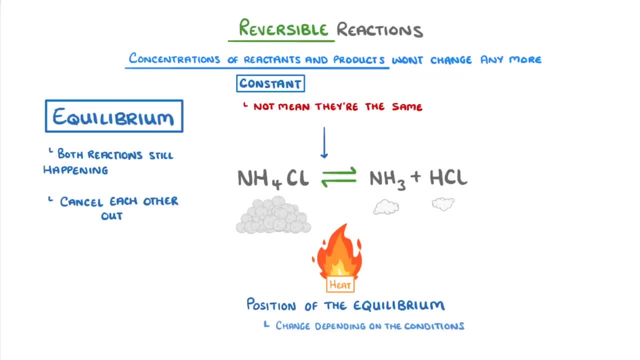 For example, adding heat to this reaction encourages the forward reaction, meaning we'll have relatively more products As the position of equilibrium moves to the right. On the other hand, if we cooled the conditions of our reaction, it would push the position of equilibrium back to the left, so it would have more ammonium chloride again. 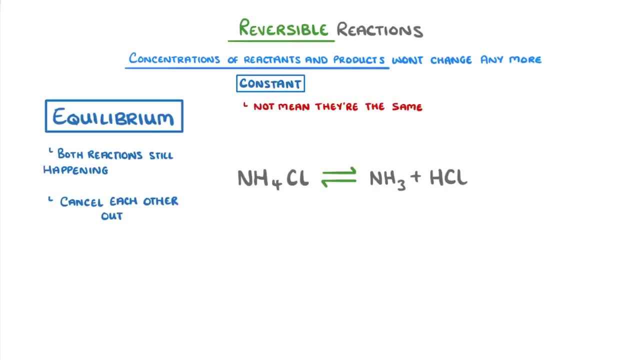 Regardless of this position, though, equilibrium can only be reached if the reversible reaction is done in a closed system, which means some kind of sealed environment from which none of the reactants or products can escape, Because if the products kept escaping, then the reaction would not be possible. 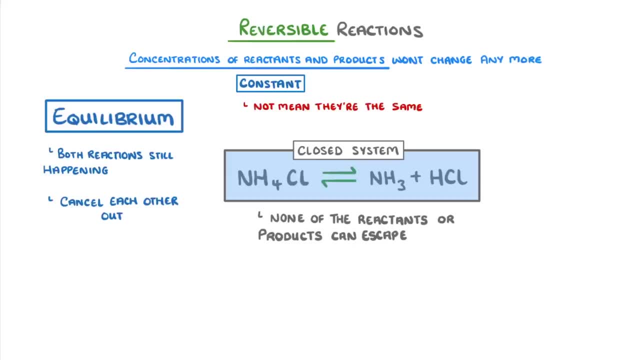 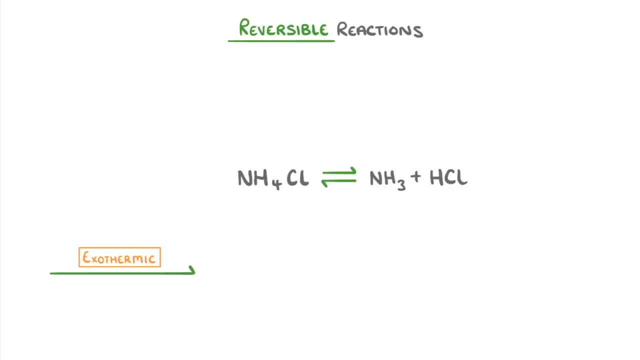 Because if the products kept escaping, then the reaction would not be possible. If the products kept escaping, then the reaction would not be possible, But if they kept escaping, it would never reach equilibrium. The last thing we need to cover is that reversible reactions are always exothermic in one direction. 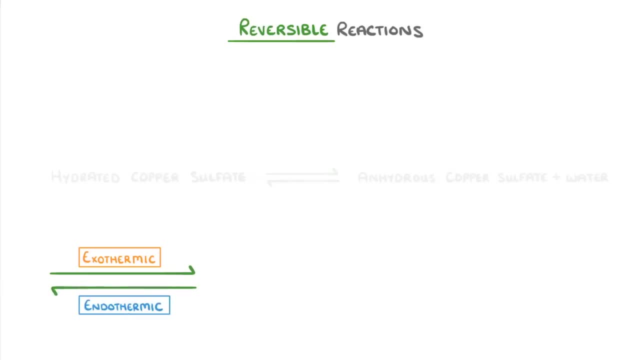 and endothermic in the other. For example, in this reaction which shows the thermal decomposition of hydrated copper sulphate to anhydrous copper sulphate and water, the forward reaction is endothermic and so the backward reaction is exothermic. 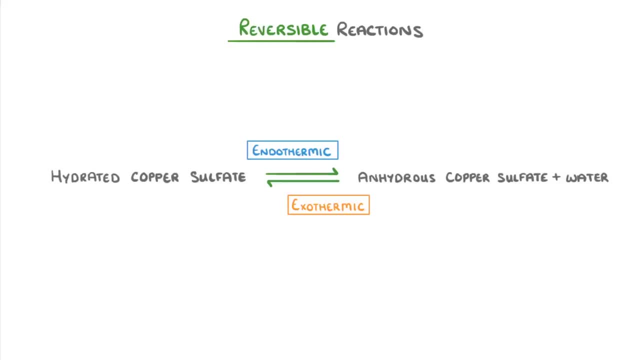 If you're not familiar with these terms: hydrated just means that water is present, and anhydrous means that there's no water. Now, because the forward reaction is endothermic, it requires heat energy from the surroundings to work. So if we were to heat some hydrated copper sulphate, which exists as blue crystals, 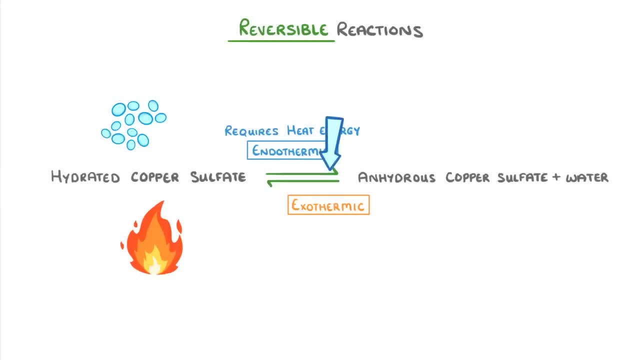 it would drive the reaction to the right, which evaporates off the water and leaves white anhydrous copper sulphate powder. If we then took away the heat and added some water to this powder, though, it would drive the backward reaction, so the equilibrium would shift to the left. 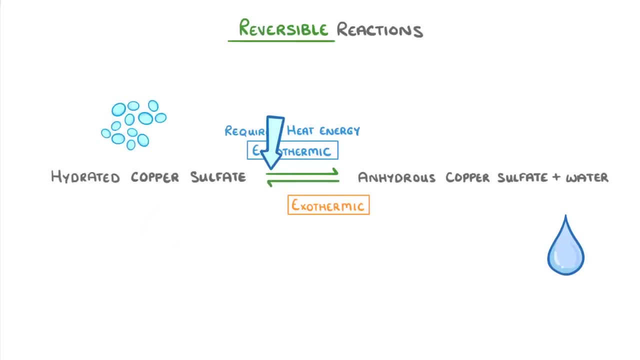 and reform our blue crystals of copper sulphate. And because this reaction is exothermic, it would re-release all of that energy it had just absorbed in the forward reaction. So to quickly recap everything, reversible reactions are those with a double arrow in the middle.